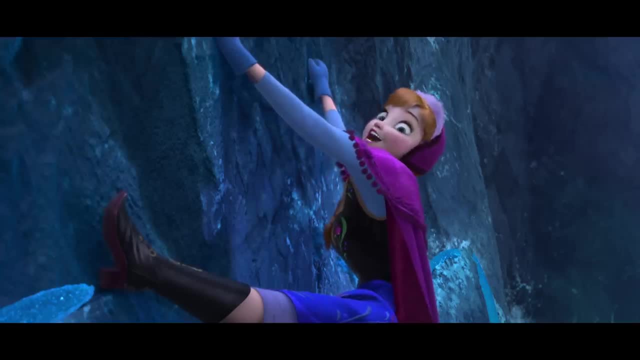 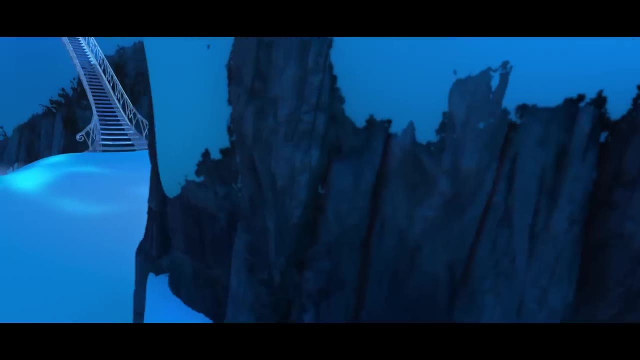 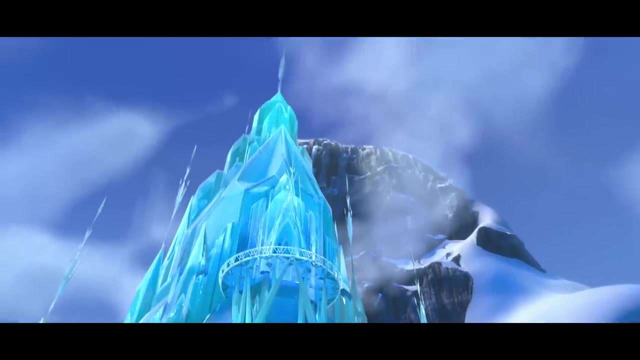 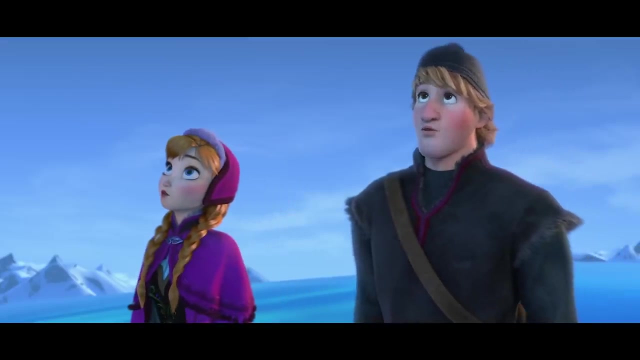 but I found a staircase that leads exactly where you want it to go. Ha-ha, Thank goodness, Catch, Thanks. That was like a crazy trust exercise. Whoa, Now that's ice. I might cry: Go ahead, I won't judge. 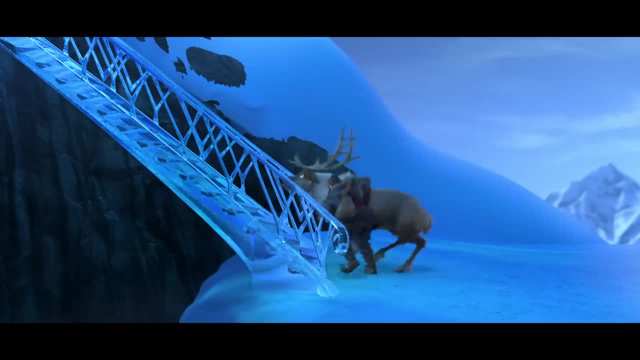 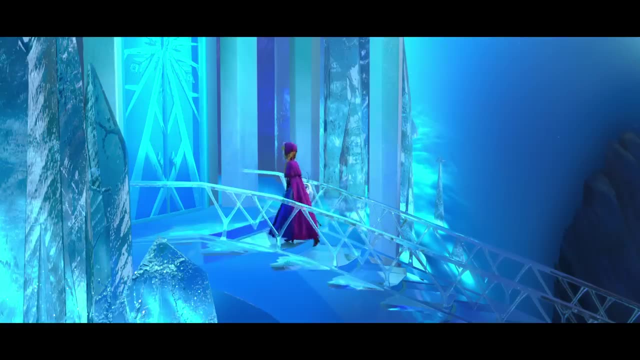 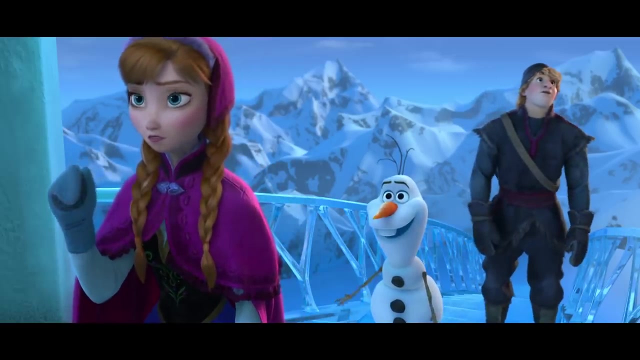 All right, take it easy. boy, Come here, I gotcha. Okay, you stay right here. buddy, Flawless, Flawless, Knock, Just knock. Why isn't she knocking? Do you think she knows how to knock? 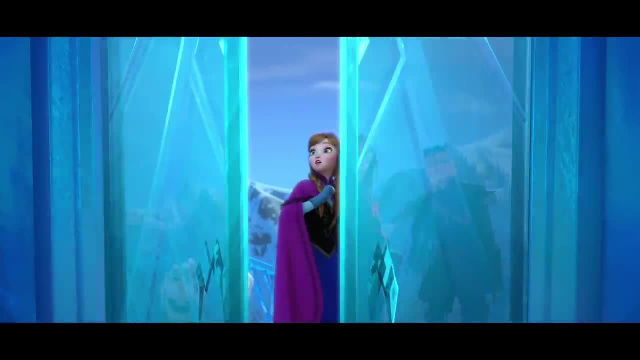 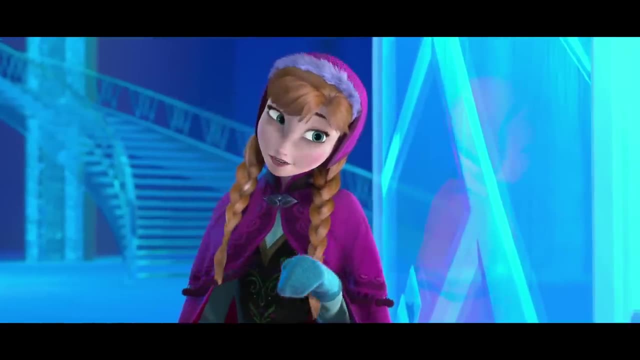 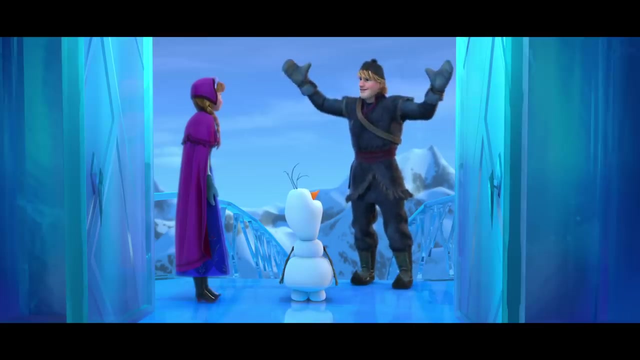 It opened. That's a first. Oh, you should probably wait out here. What Last time I introduced her to a guy? she froze everything, But but oh, come on, It's a palace made of ice. Ice is my life. Bye, Sven. 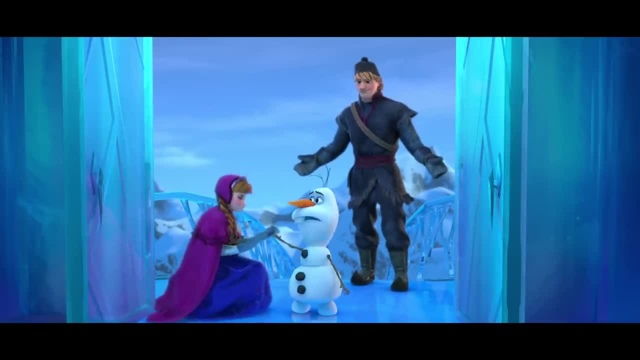 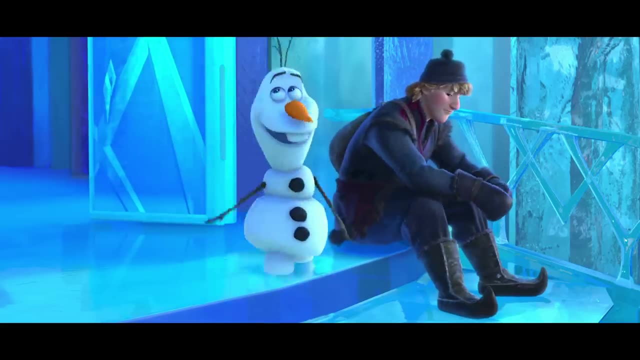 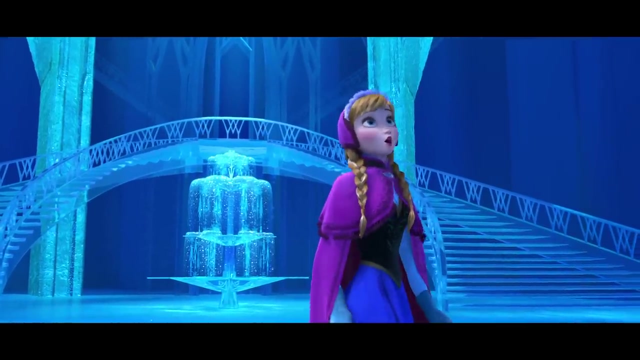 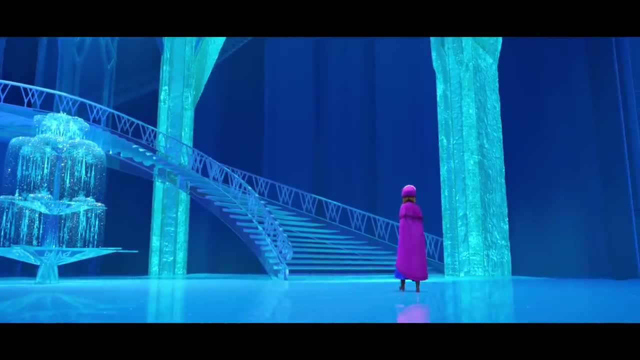 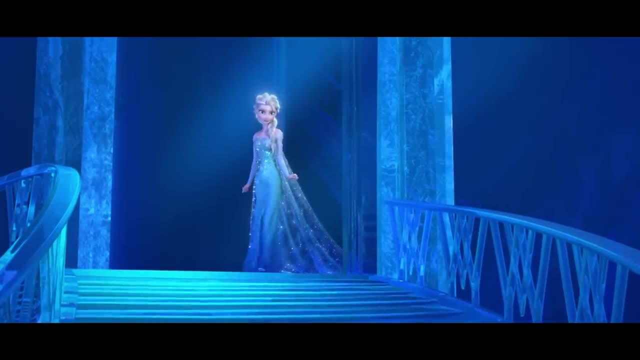 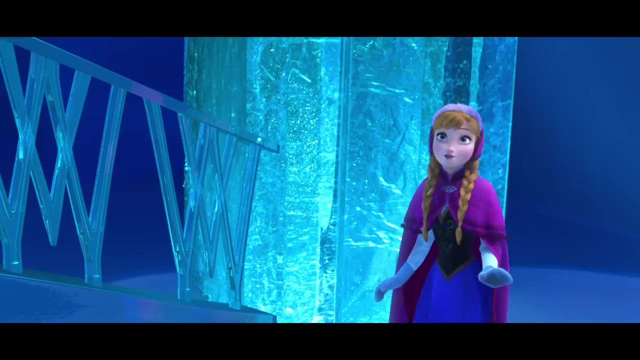 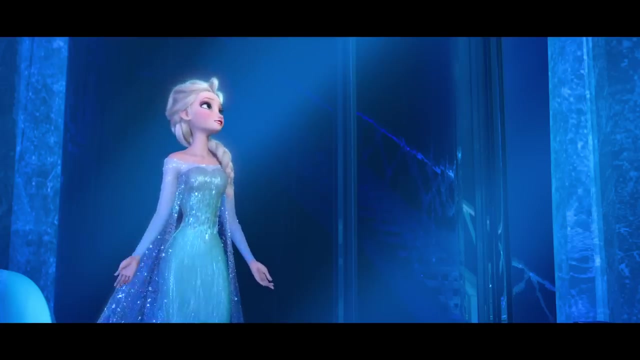 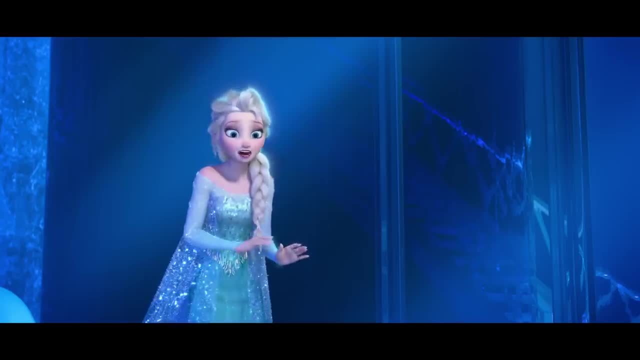 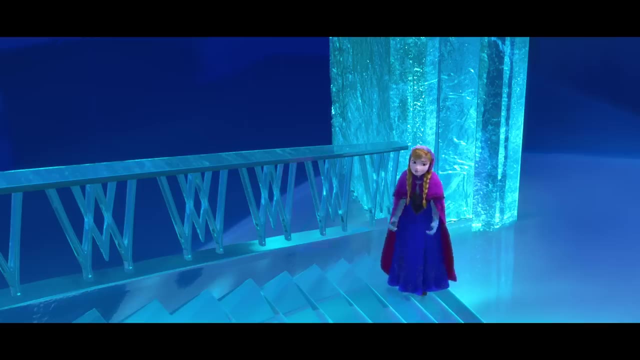 Elsa, you look different. It's a good difference, And this place, It's amazing. Thank you, I never knew what I was capable of. I'm so sorry about what happened. If I'd have known. No, no, no, no. 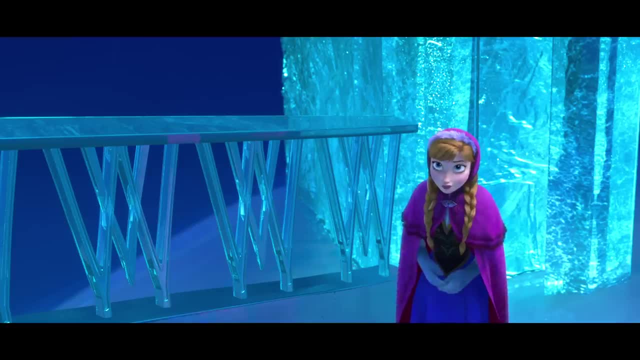 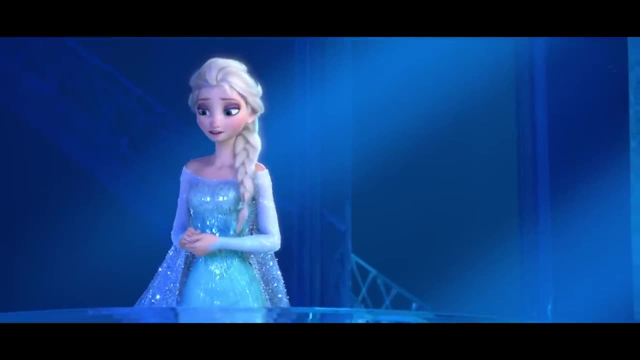 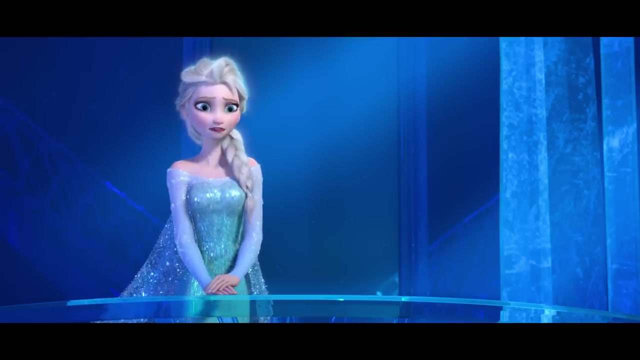 It's okay. You don't have to apologize, Arendelle, So do you? No, Anna, I belong here Alone, Where I can be who I am without hurting anybody. Actually, about that. Wait, what is that? Hey, I'm Olaf, and I like warm hugs.